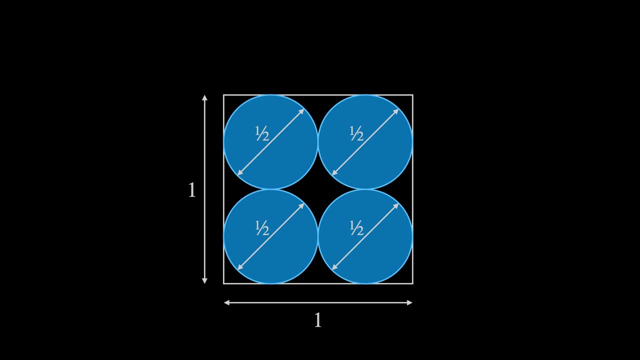 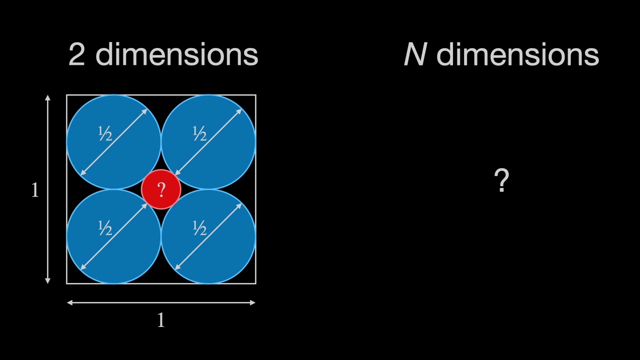 diameter one half, so they fit exactly inside the square. This leaves an empty region in the center where we place an inner circle. We are interested in the size of the inner circle. We will consider generalizations of this figure in three, four and more dimensions, and we will 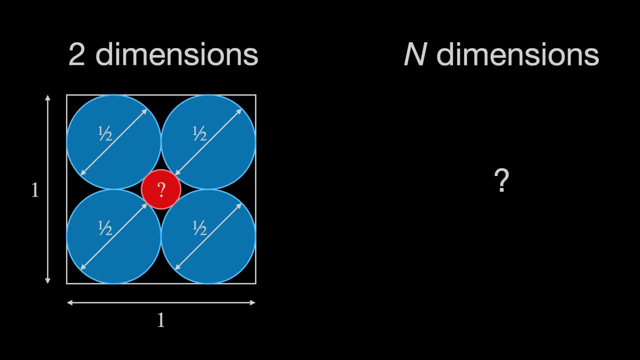 be interested in the size of the inner circle, or hyposphere as it is called, in higher number of dimensions. The question we ask is what happens to the size of the inner hyposphere as the number of dimensions grow? The surprising answer is that the inner hyposphere grows without. 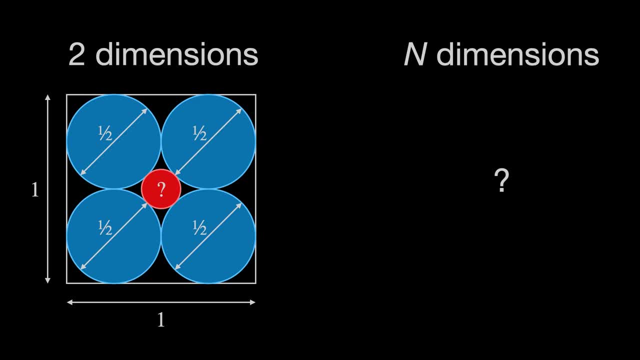 bound Already in 10 dimensions. it is so big that it stretches outside of the hypercube that it is not visible in the inner circle. The problem with the inner hyposphere is that contains the blue hypospheres, In the two-dimensional case, an inner circle of 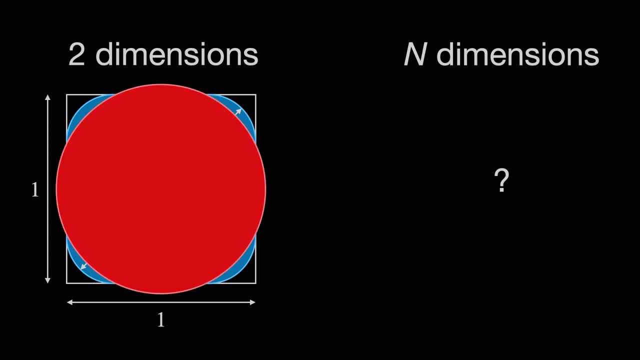 that size would have to overlap with the blue circles, but we don't allow any overlap. So how can this happen in ten dimensions? How can the inner hyposphere extend outside the hypercube when it is also between the blue hypospheres, which? 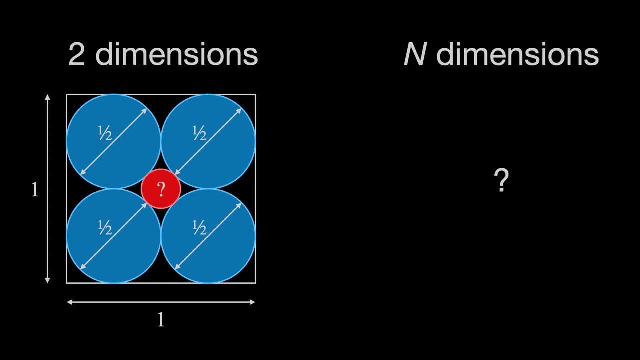 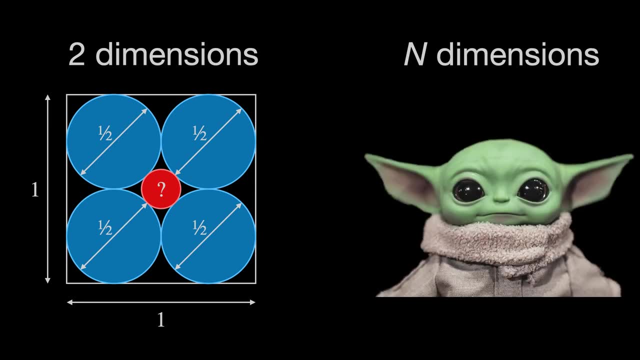 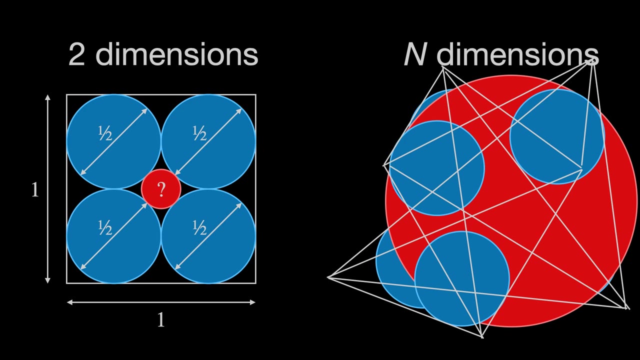 are all inside of the hypercube. A mathematician may explain it using pure equations. An alien might be able to visualize it directly in ten dimensions. An artist may draw a crazy interpretation like this, illustrating the strange fact that the red hyposphere extends outside the boundaries. But crazy. 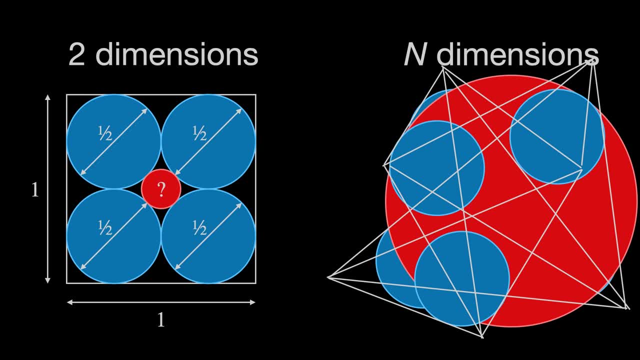 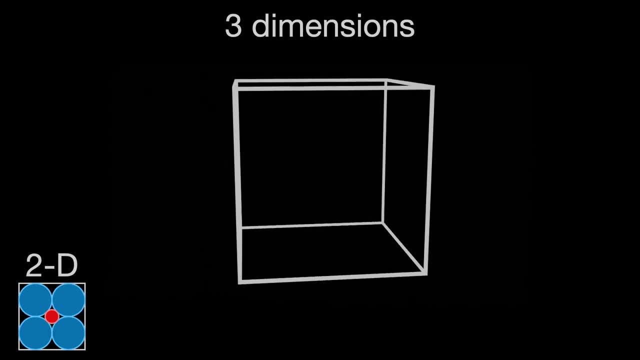 as it is, this figure is not based on the underlying math and it doesn't explain anything. Let's look at the situation in three dimensions. We create a cube with side length 1.. Inside the cube, we have a cube with a. 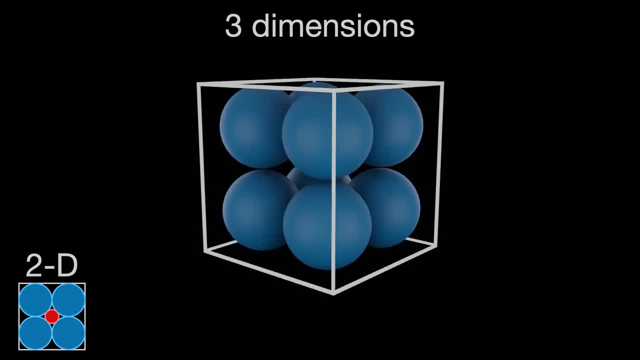 diameter 1.5.. We put eight blue spheres with diameter 1.5, one towards each corner. In the empty space in the center we put an inner sphere that touches the blue spheres. How big is the inner sphere in this 3D case compared to the 2D case? 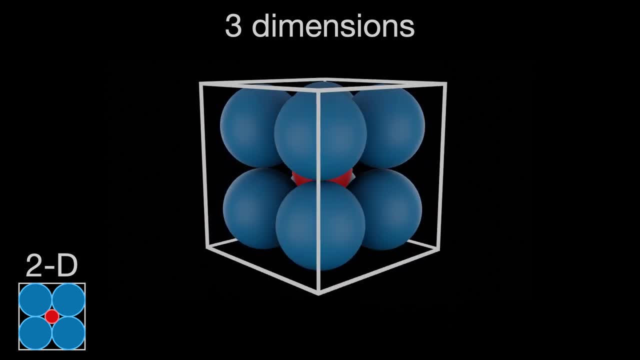 Can we understand this visually? To do this, we make a two-dimensional cut through the cube like this: The cut follows two opposite edges of the cube and goes through its center. The cut only passes through four of the blue spheres and they appear as circles. The inner sphere also appears as 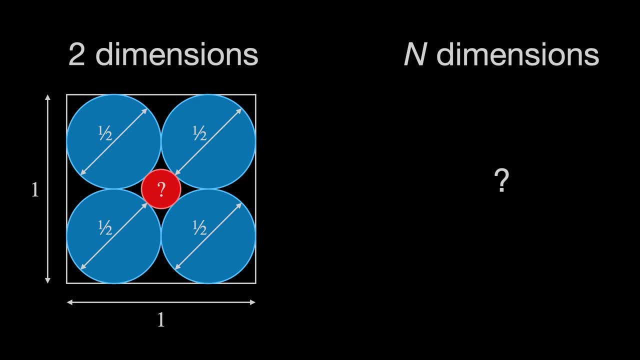 bound Already in 10 dimensions. it is so big that it stretches outside of the hypercube that it is not possible to measure the size of the inner hyposphere. It is not possible to measure the size of the inner hyposphere that contains the blue hypospheres In the two-dimensional case. 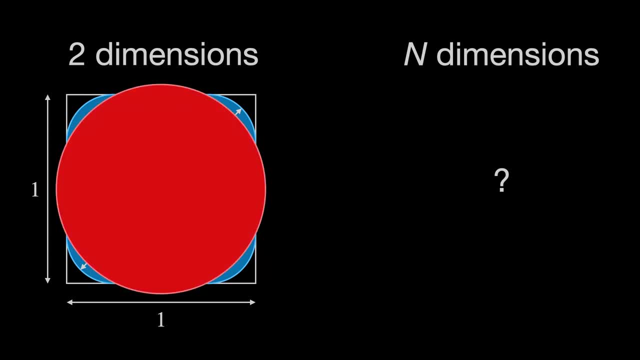 an inner circle of that size would have to overlap with the blue circles, but we don't allow any overlap. So how can this happen in 10 dimensions? How can the inner hyposphere extend outside the hypercube when it is also between the blue hypospheres which are all inside of the hypercube? 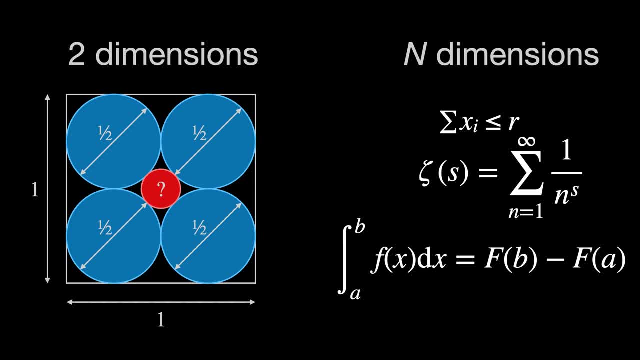 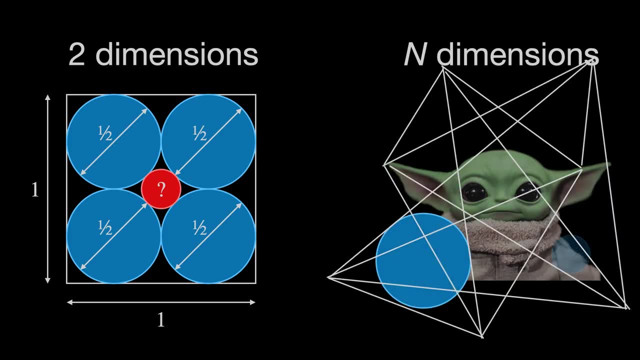 A mathematician may explain it using pure equations. An alien might be able to visualize it directly in 10 dimensions, but it is not possible to measure the size of the inner hyposphere when in 10 dimensions. An artist may draw a crazy interpretation like this, illustrating the 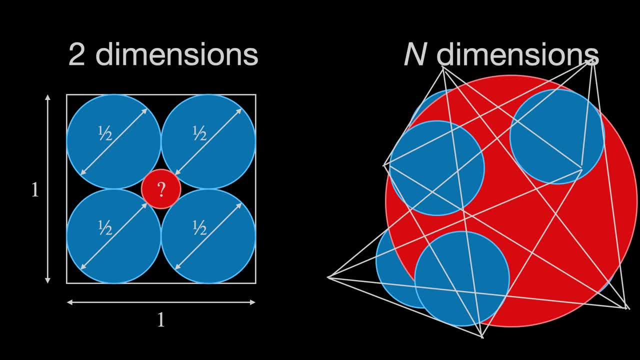 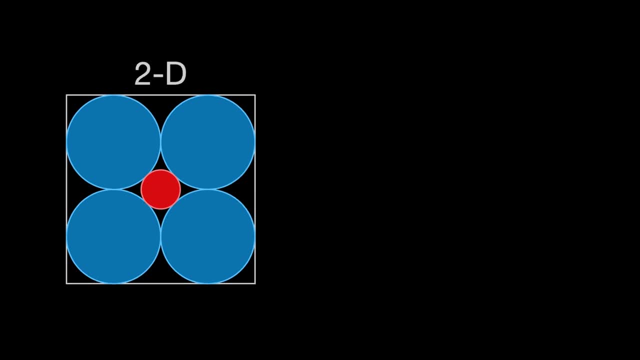 strange fact that the red hyposphere extends outside the boundaries. But crazy as it is, this figure is not based on the underlying math and it doesn't explain anything. Let's look at the situation in three dimensions. We create a cube with side length 1.. 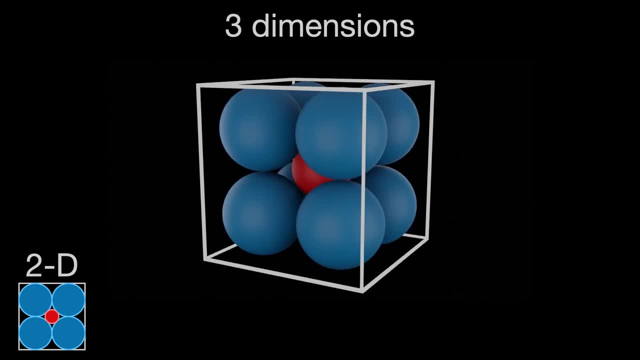 Inside the cube we put eight blue spheres with diameter one half one towards each corner. In the empty space in the center we put an inner sphere that touches the blue spheres. How big is the inner sphere in this 3D case compared to the 2D case? Can we understand this? 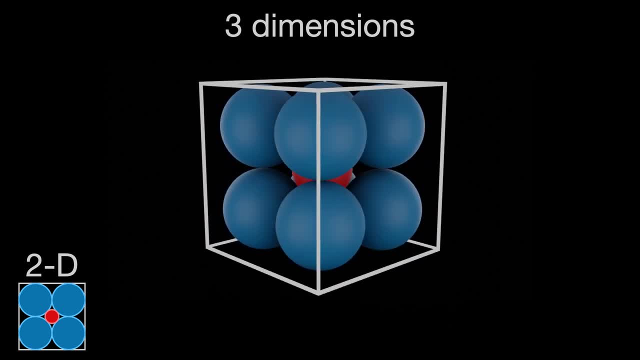 visually. To do this, we make a two-dimensional cut through the cube like this: The cut follows two opposite edges of the cube and goes through its center. The cut only passes through four of the blue spheres and they appear as circles, The inner. 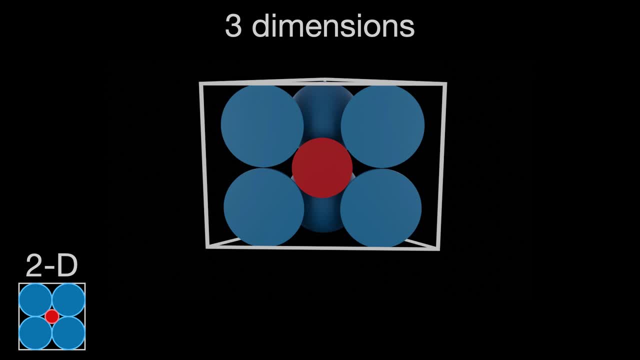 sphere also appears as a circle in the cut. Note that the cut of the 3D figure is somewhat similar to the 2D case, but there is an important difference. The cut creates a rectangle which is stretched out such that there is more space between the blue circles in one direction. 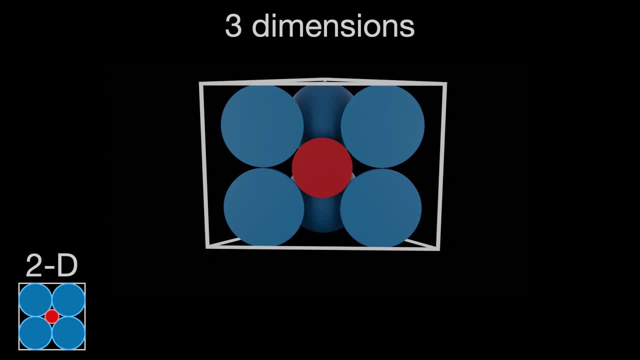 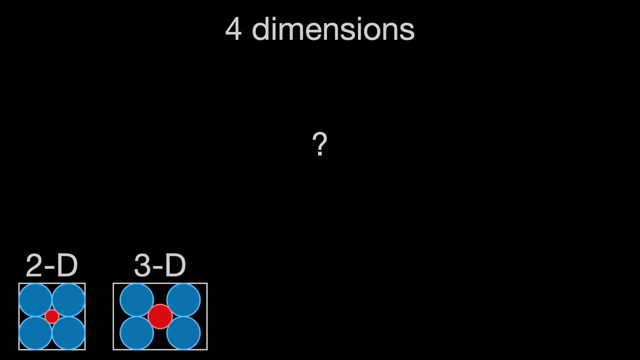 This extra space allows the inner sphere to be bigger in the 3D case compared to the 2D case. What happens in 4D? It is difficult to visualize four dimensions, but we can make a two-dimensional cut in much the same way as we did in 3D and look at that. 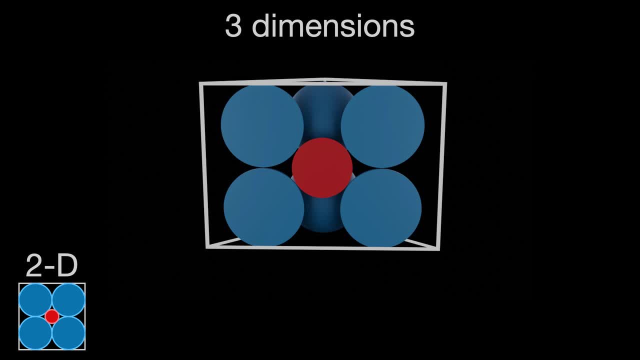 a circle in the cut. Note that the cut of the 3D figure is somewhat similar to the 2D case, but there is an important difference. The cut creates a rectangle which is stretched out such that there is more space between the blue circles. 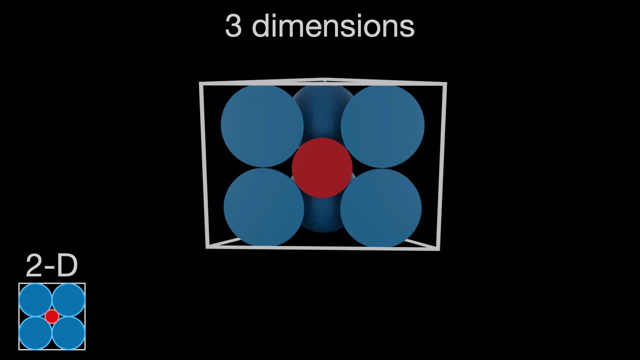 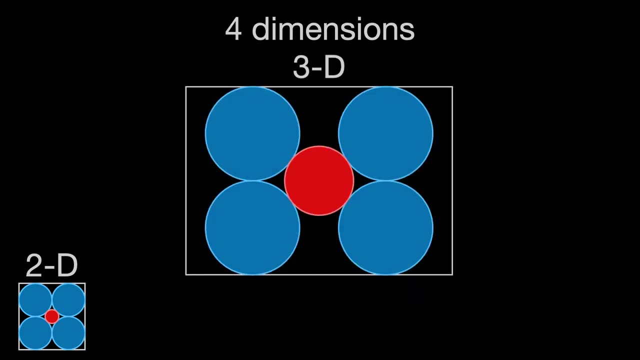 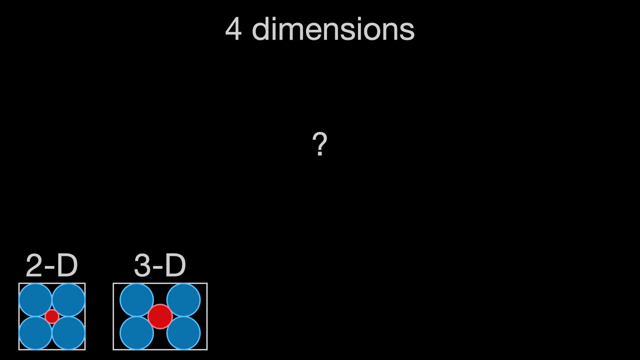 in one direction. This extra space allows the inner sphere to be bigger in the 3D case compared to the 2D case. What happens in four dimensions? It is difficult to visualize four dimensions, but we can make a two-dimensional cut in much the same way as we did in 3D and 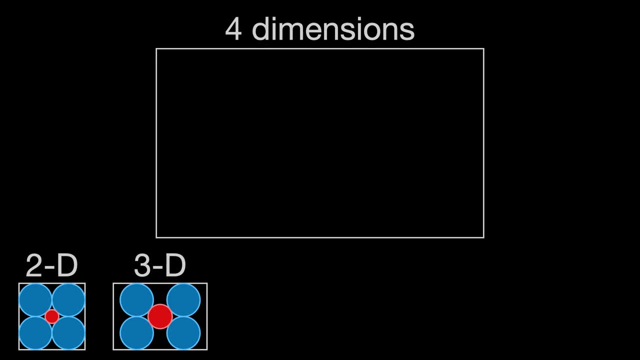 look at that. Just as in the 3D case, the cut follows two opposite edges of the 4D hypercube and goes through its center. In this cut, four of the blue hyperspheres are visible, as well as the inner hypersphere, So the cut looks much like. 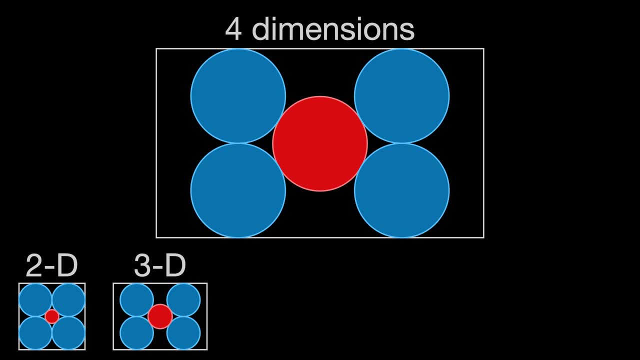 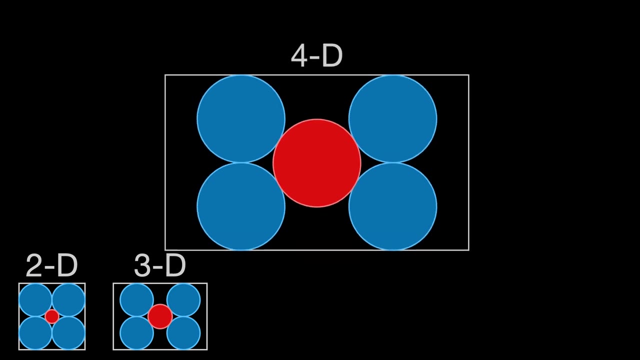 the cut from 3D, but it is stretched a bit more. This is because it contains the diagonal of the hypercube, which is longer than the diagonal in the 3D cube. Because of this additional stretching, there is even more space in the middle, allowing the inner hypersphere to be even bigger. 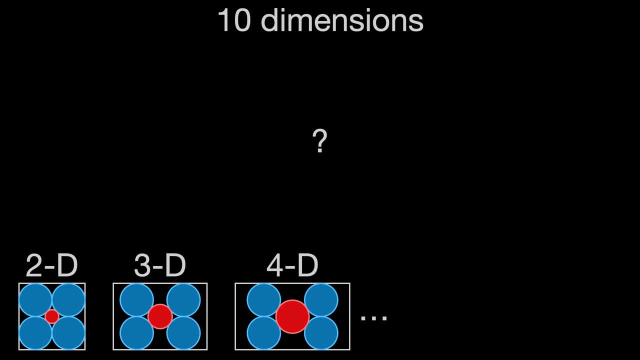 The same technique works in any number of dimensions. Let's look at the 2D cut of the 10-dimensional figure. The hypercube appears as a stretched rectangle in the cut. It is stretched quite a lot since it contains the hyperdiagonal of the 10-dimensional cube. Four of the blue. 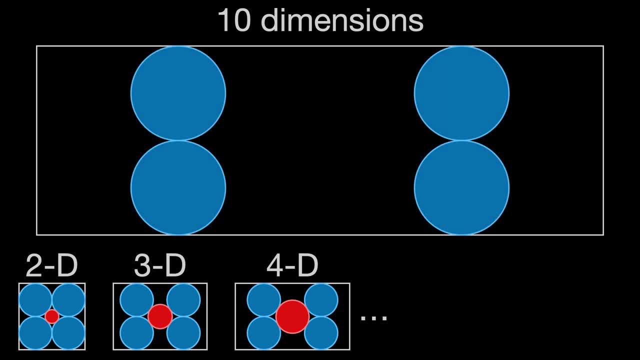 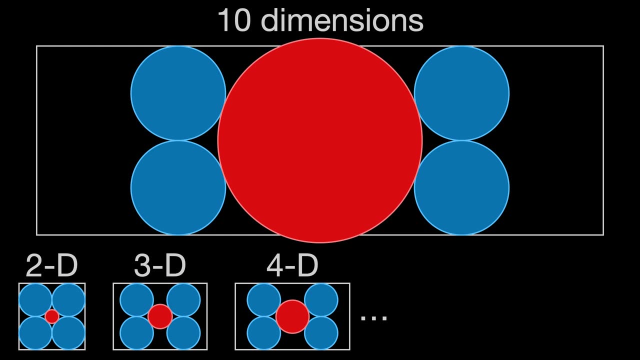 hyperspheres show up as a circle in the cut. Note how far apart they are spaced in the diagonal direction of the hypercube. Finally, we can see the size of the inner hypersphere, how it extends outside of the boundaries of the hypercube. We can see why this happens. It is because there is a lot of room. 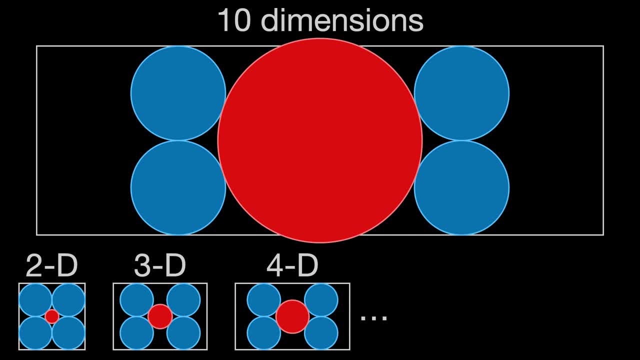 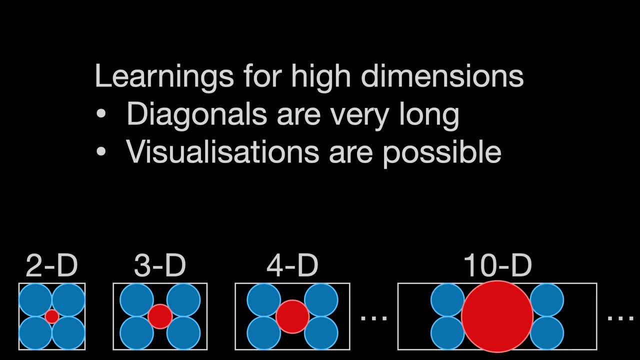 between the blue hyperspheres in the diagonal direction. What can we learn from this? A direct learning is that diagonals are longer than sides and that this effect becomes stronger the more dimensions there are. The longer distance along the diagonal comes, because you have to travel along many dimensions simultaneously.